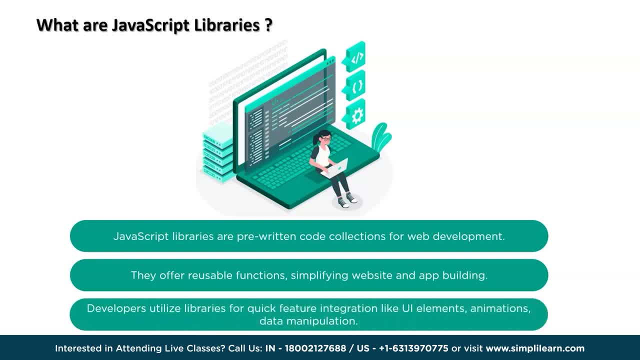 These libraries contain reusable functions and methods that help simplify and speed up the process of building websites and web applications. Instead of creating code from scratch, developers can use these libraries to create in-corporate features like animations, user interface components, data manipulation, etc. 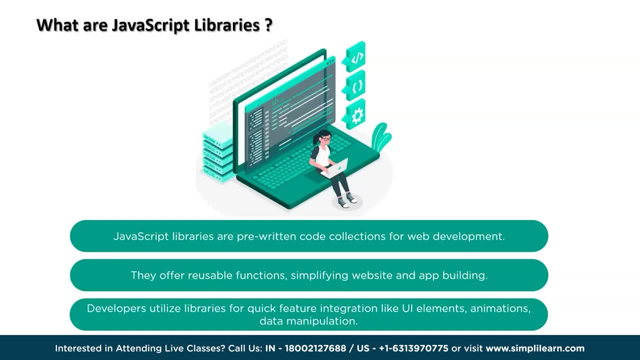 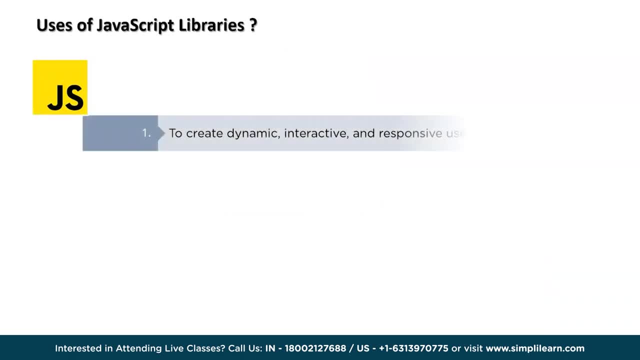 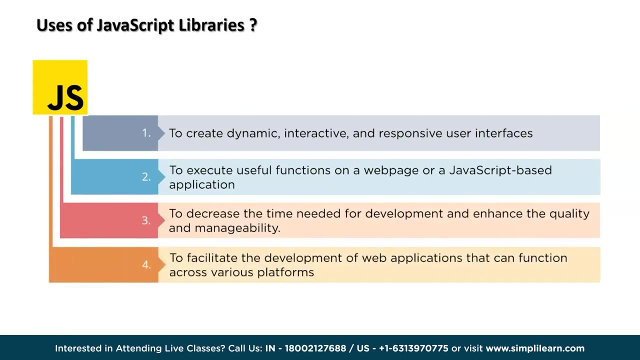 So this was about what are JavaScript libraries? Alright, now let's understand uses of JavaScript libraries. Let's start So. the first use is to create dynamic and interactive and responsive user interfaces. Second is to execute useful functions on a web page or a JavaScript-based application. 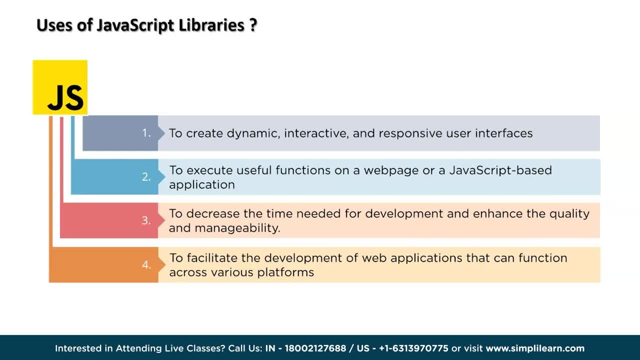 such as animation, visualization, data validating input and manipulating content. Third use is to decrease the time needed for development and enhance the quality and manageability of the code. And the fourth use is to facilitate the development of web applications that can function across. 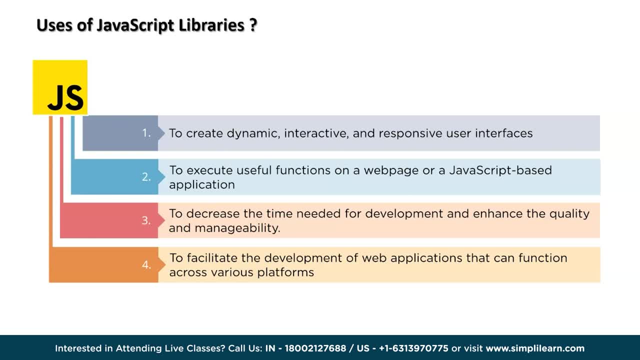 various platforms. And the last use is to make JavaScript libraries more accessible to users, ensuring compatibility with diverse browsers and devices. So these are the four uses that we have mentioned, But, yeah, definitely there are many other uses of JavaScript libraries as well. 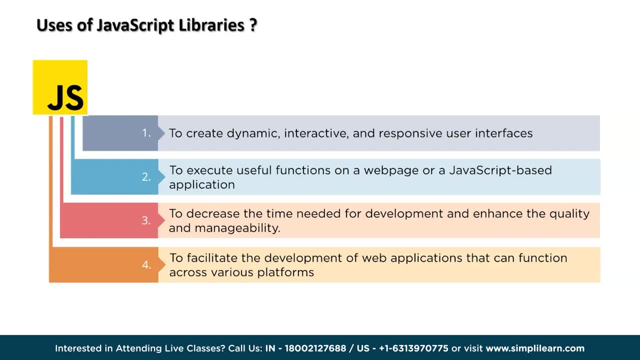 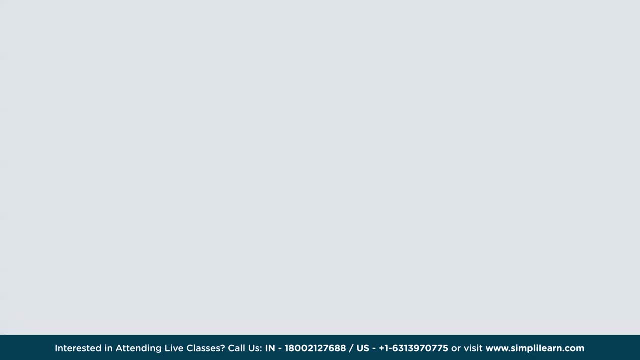 Alright, now we will discuss five new JavaScript libraries that you can use in your next project, So let's start with the first one, which is Animatejs. Animatejs is a powerful animation library that enables developers to create smooth and eye-catching animations for their websites and web applications. 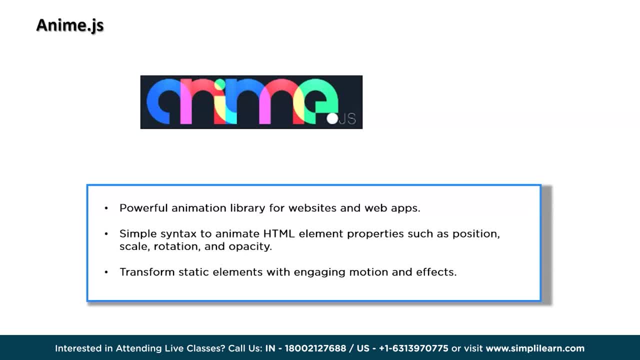 It provides a simple and intuitive way to create smooth and eye-catching animations. However, it's a simple and intuitive syntax for animating various properties of HTML elements, such as position scale, rotation and opacity. With Animatejs, developers can easily bring static elements to life and enhance user experience. 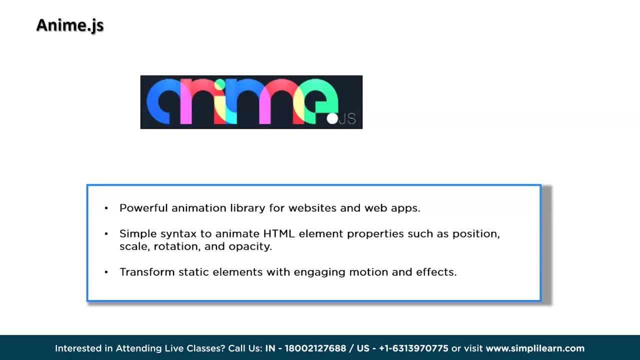 by adding engaging animations. Moreover, Animatejs exhibits versatility by seamlessly working with an array of elements. It seamlessly interfaces with CSS properties, SVG, DOM attributes and even JavaScript objects. This compatibility allows for the creation of a variety of animations. Animatejs is a powerful animation library that enables developers to create smooth and 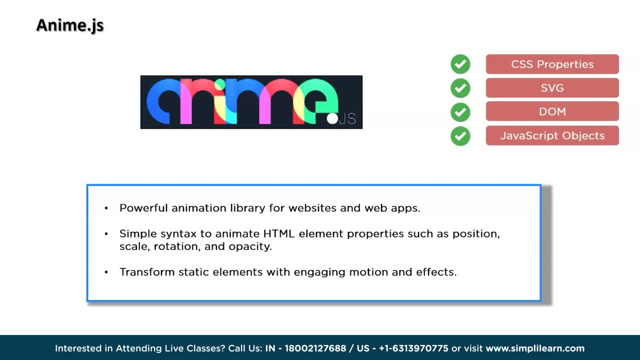 eye-catching animations for their websites and web applications. Animatejs is a powerful animation library that enables developers to create smooth and eye-catching animations for their websites and web applications. It seamlessly interfaces with CSS properties, JS and JavaScript. This compatibility allows for the creation of intricate animations with remarkable ease. 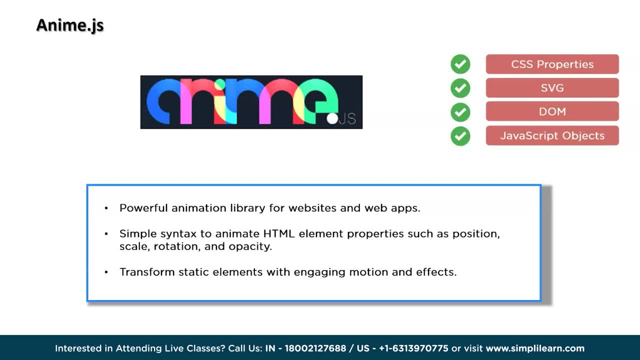 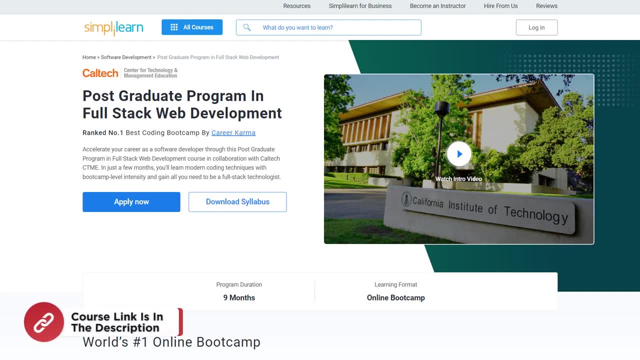 and optimal performance. If you're working on a project on JavaScript, then this is one of the most essential JavaScript libraries that you can use. Also, if you're aiming to become a full-stack web developer, then try our Postgraduate Program in Full-Stack Web Development. 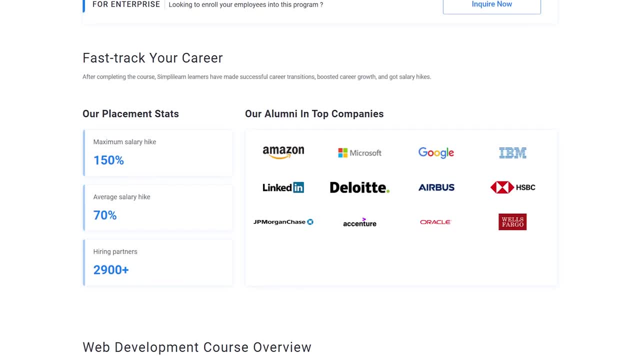 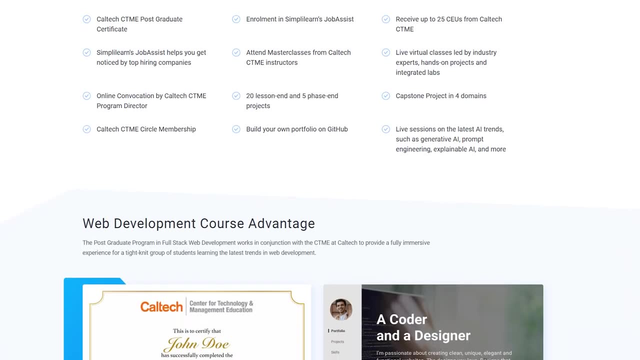 This program will give you the foundation for building full-stack web apps using the Java programming language. You will begin with the basics of JavaScript and then venture into some of the more advanced JavaScript programming languages. Enjoy Good luck. Bye-bye. advanced concepts like Angular, Spring Boot, Hibernate, JSP and MVC. 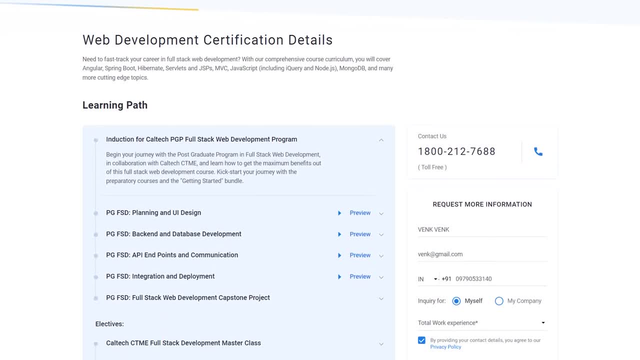 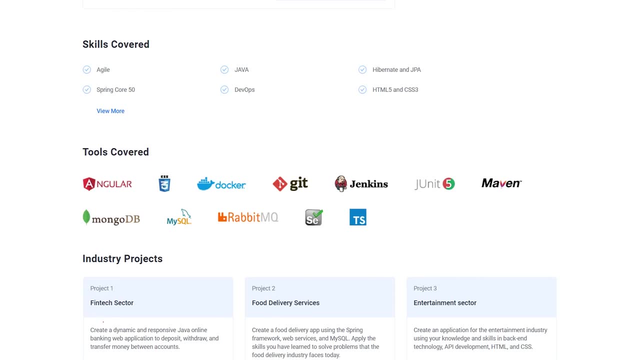 Now is a perfect time to get started on your career as a full stack web developer. To find the details of Simply Learn's postgraduate program in full stack web development, check the link in the description box below. It could be the ideal solution to help you build your career in the right direction. 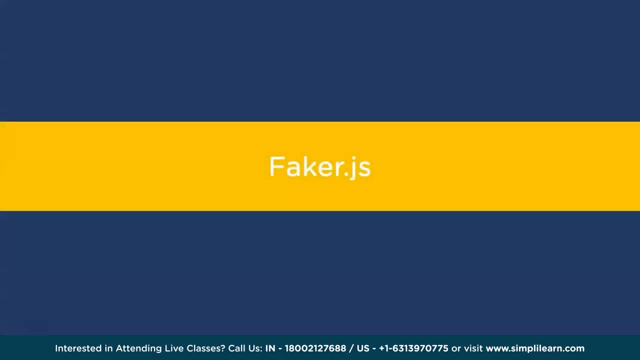 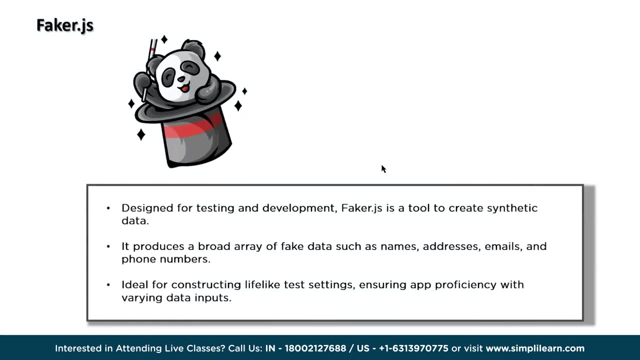 Alright, now let's move on to the second library, which is fakerjs. So, fakerjs is a library designed to generate fake data for testing and development purposes. It can generate a wide range of fake data, including names, address and phone numbers, email addresses and more. 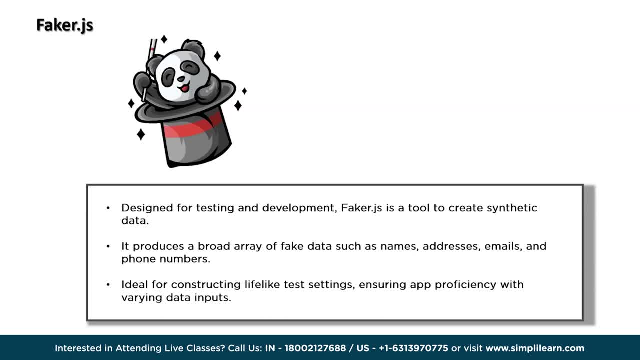 This is incredibly useful for creating realistic test environments without using real user data. Developers can use fakerjs to simulate various scenarios and ensure applications handle different data inputs effectively. Fakerjs is like a super important tool for making test situations feel real. Developers can make situations and then test how well their apps work. 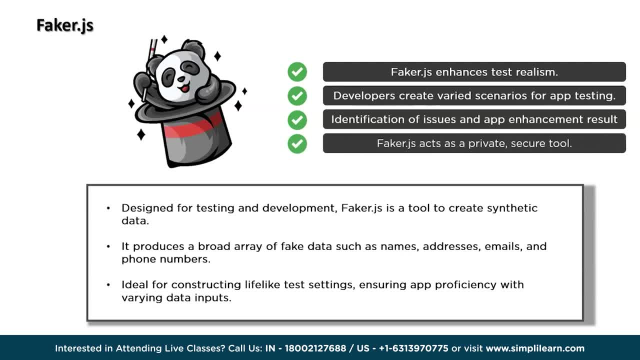 This helps find the problems and make the apps better. It's kind of like having a secret weapon for developers. They can use fakerjs to create situations that look and act like real data, but without using real people's info. This keeps things private and safe. 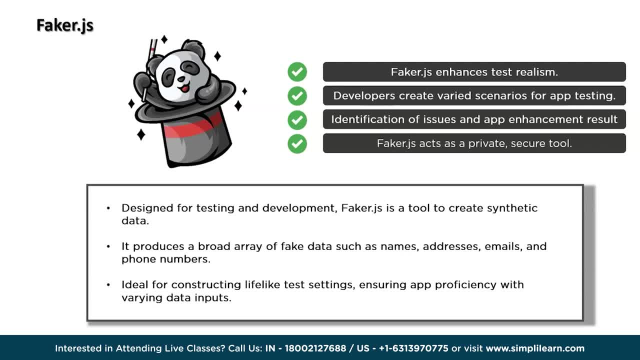 So, to put it simply, fakerjs is a must-have tool for developers. It lets them to pretend to use real data without causing any privacy problems. So this was about fakerjs. You can try this library while building your JavaScript project. Thanks for watching. 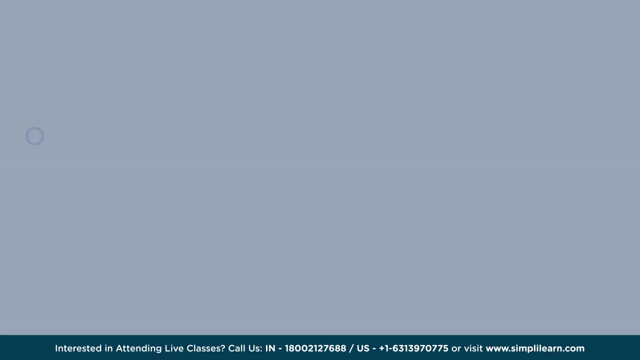 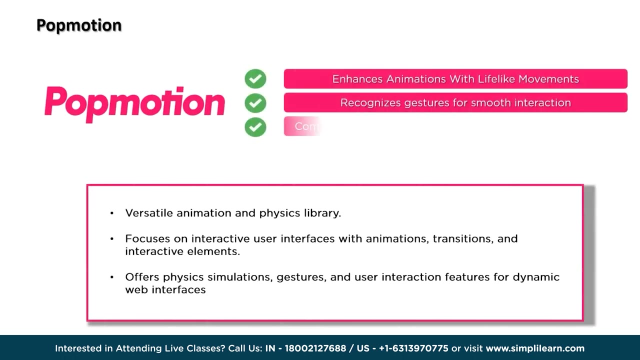 All right. now moving on to the next library, which is PopMotion. So PopMotion is a versatile animation and physics library that focuses on creating interactive and engaging user interfaces. It offers tools for creating animations, transitions and interactive elements using a straightforward API. 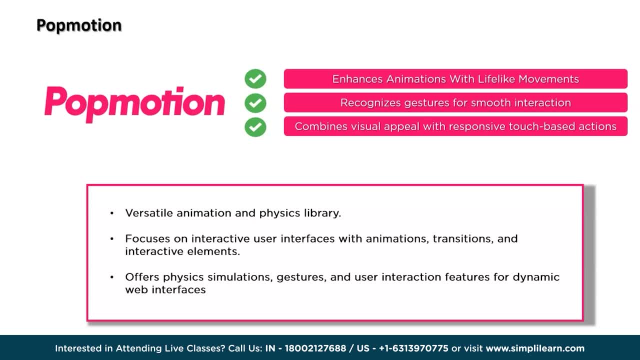 PopMotion also includes features for handling physics simulations, gestures and user interactions, making it a great choice for building dynamic and lively web interfaces. But wait, there's more. PopMotion isn't just about making things look pretty. it's also great at handling. 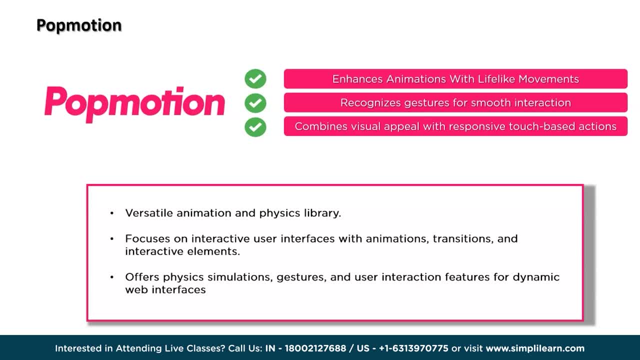 the way things move in a natural way, like how a ball bounces or a spring stretches. This makes animations feel more realistic and lifelike. And guess what? It's not just about clicking and moving things. PopMotion understands gestures too. 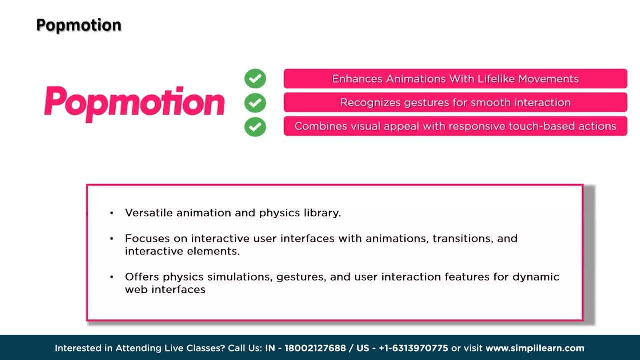 Think of swiping, tapping and other ways you interact with your phone. This library can handle those actions smoothly, making websites feel like they're responding to your touch. So this is one of the most important features And I hope you found this video helpful. 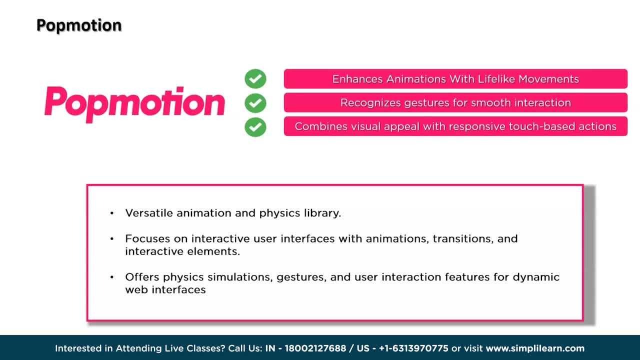 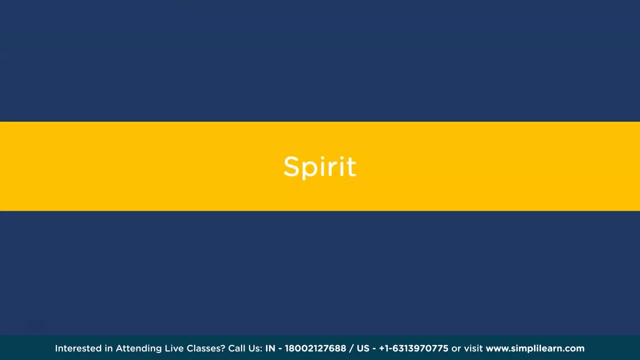 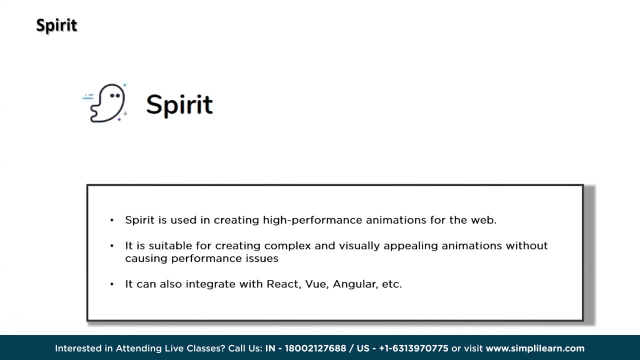 I'll see you in the next one. PopMotion is a lightweight animation library that specializes in creating high-performance animations for the web. It is designed to be efficient and optimized for smooth animation rendering, making it suitable for creating complex and visually appealing animations without causing performance. 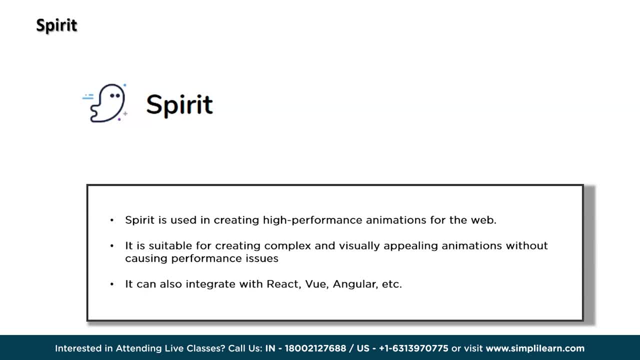 issues. Spirit provides an API for creating animations using a timeline-based approach. It can also be used to create animations that are easy to use. It can also integrate with React, Vue, Angular, etc. It is like Super Skill Magician for web animations. 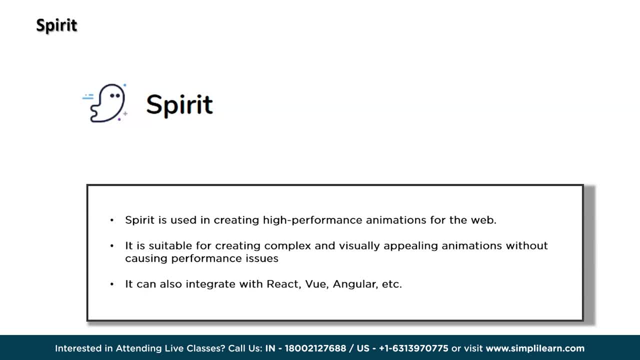 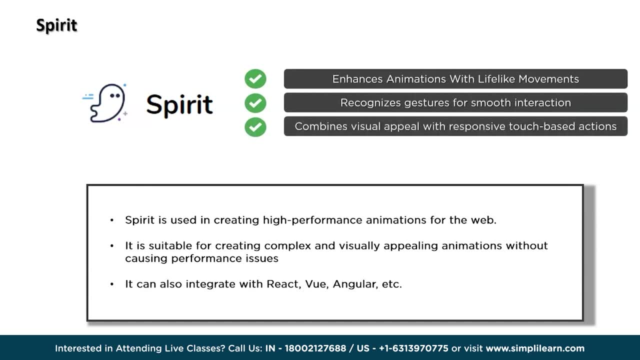 It's a small and efficient library that's all about making animations on the web run super smoothly. It is designed in a way that it's really good at making animations look awesome without making your computer struggle. One cool thing about Spirit is how it organizes animation. 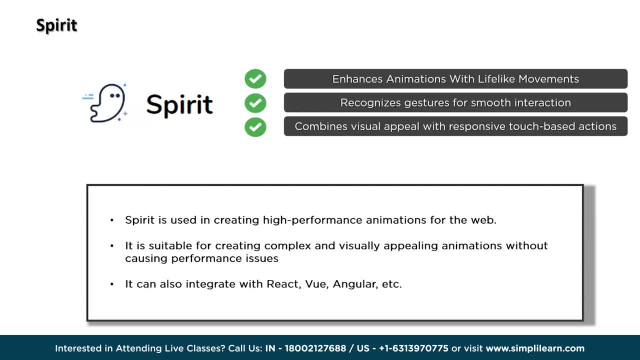 It uses something called a timeline-based approach. This means you can plan out how different animations happen at different times. It's kind of like choreographing a dance: You decide when each move should happen to create a beautiful sequence. Spirit lets developers do the same thing with animations on websites. 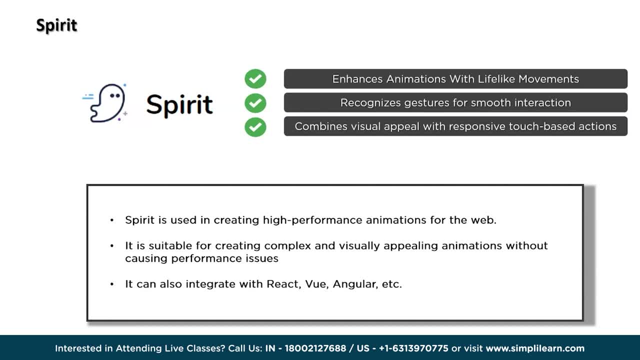 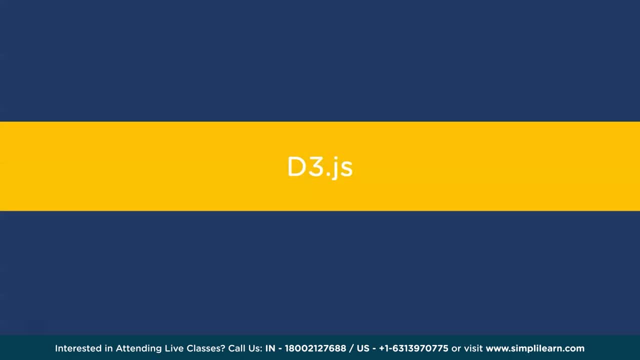 Alright, So this was about the Spirit library. Now coming to the next library, which is D3.js. So D3.js, that is Data Driven Documents. So Data Driven Documents library is a powerful data visualization library that enables developers to create interesting animations. 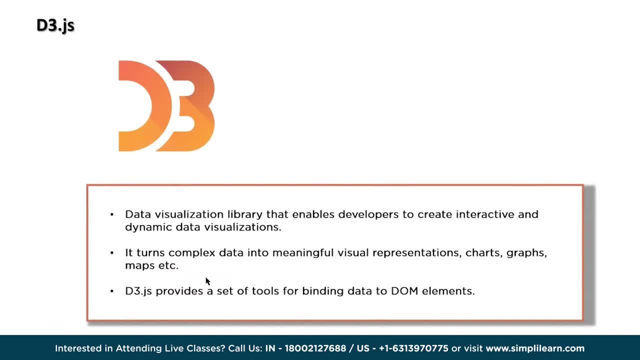 It has interactive and dynamic data visualizations using HTML, SVG and CSS. It's particularly well suited for displaying complex datasets and turning them into meaningful visual representations, such as charts, graphs, maps and more. D3.js provides a set of tools for binding data to DOM elements and updating the visualizations. 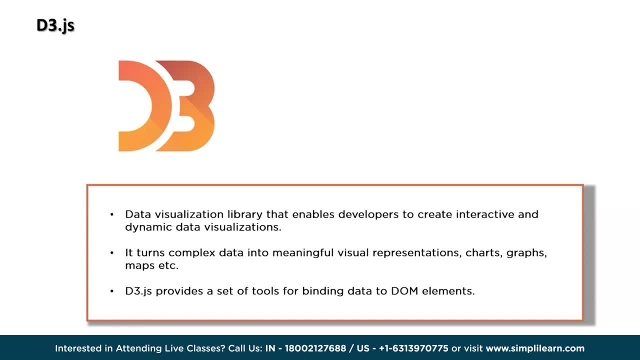 as the data changes. D3.js is like a wizard that can make complex data look simple and understandable. You know, When you have a lot of numbers and you're not sure what they mean, D3.js can take those numbers and create charts, graphs and even maps that make it easy to see patterns and 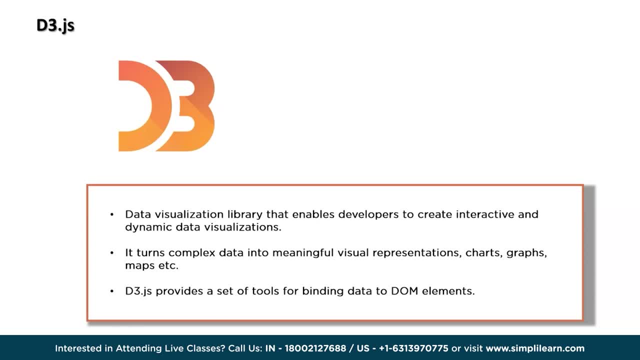 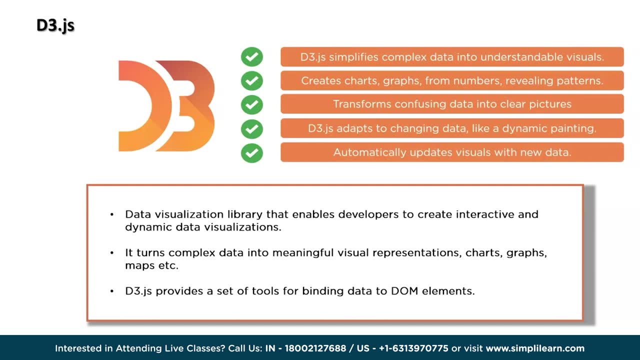 trends. It's like turning a confusing table or puzzle into a clear picture. One of the cool things about D3.js is that it's not just a one-time thing. It's like having a magical painting that changes as the data changes. Let's say, you are tracking the weather each day. 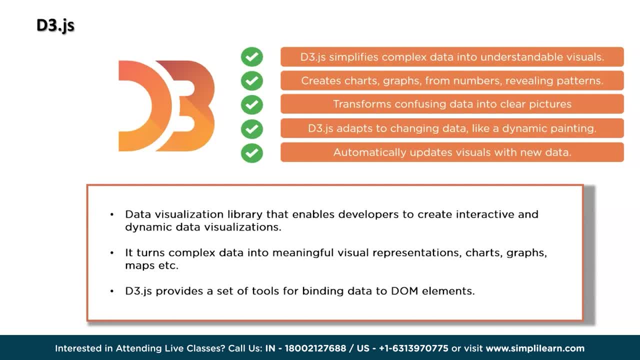 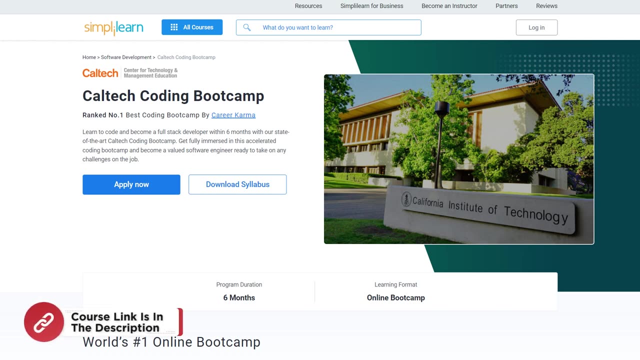 So D3.js can automatically update the chart to show the new weather data without you having to redraw everything. So this was about D3.js. It is also another interesting JavaScript library. Also, guys, if you want to become unstoppable at coding, then you can join Caltech Coding. 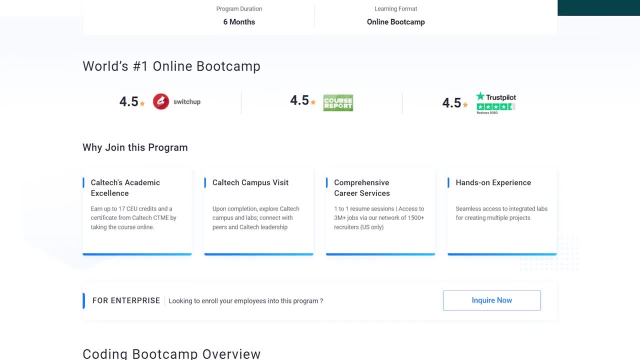 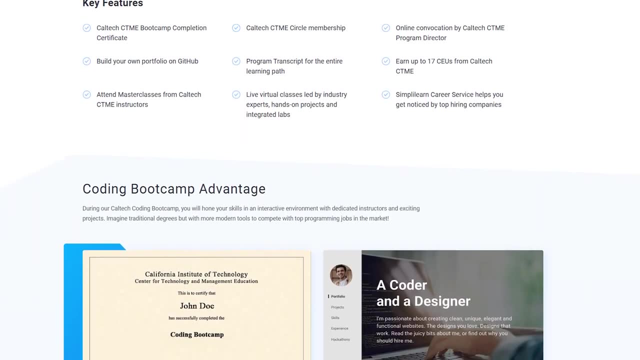 Bootcamp by SimplyLearn: Master front-end and back-end Java technologies, progressing basics to advanced full-stack web development. learn Angular, Spring Boot, Web Services, JSPs and MongoDB to kickstart your career. Enjoy key features like Caltech, CTME, Bootcamp completion certificates and more. 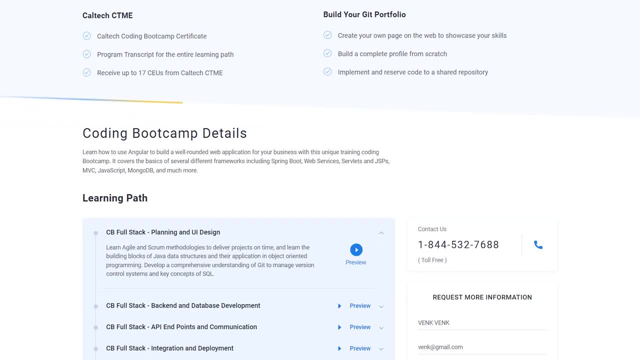 You can also join Caltech Coding Bootcamp by simplylearn Master front-end and back-end Java technologies, progressing basics to advanced full-stack web development. learn Angular, Spring Boot, Web Services, JSPs and MongoDB to kickstart your career. 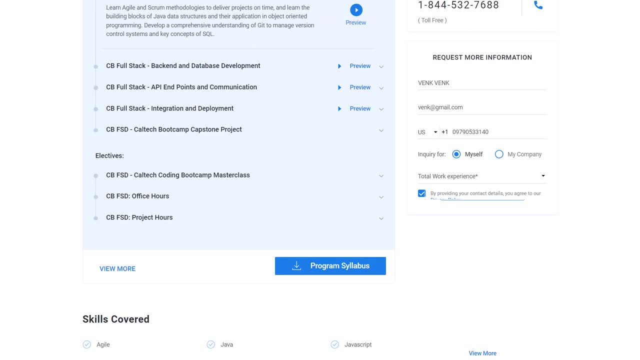 You can also join Caltech Coding Bootcamp by simplylearn. Yeah, now let's take a look at some other cool other things that you can also add to your Java design project. You can add some Coding software as well. Watch and learn another ones as well. 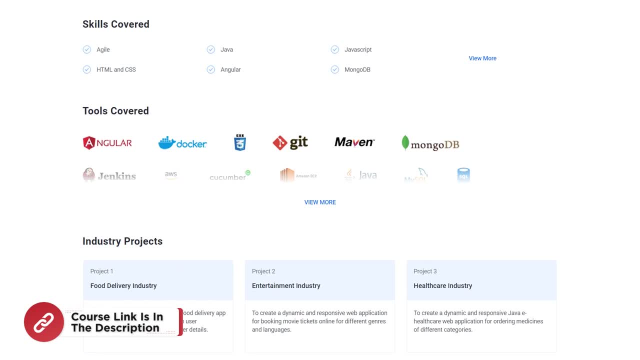 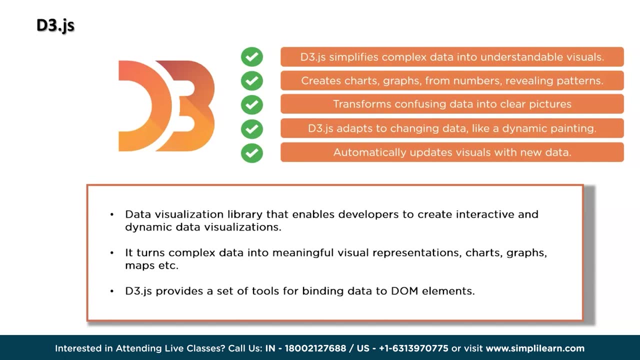 So this is about the JavaScript libraries, the five new JavaScript libraries that you can include in your next project. So we have come to the end of this video. So, in this ever-evolving world of web development, staying up-to-date with the latest tools and 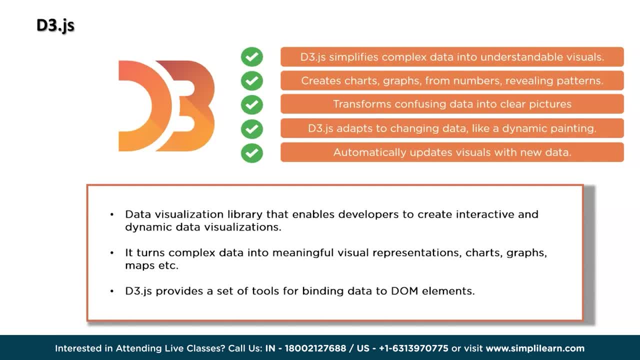 technologies is key to crafting exceptional digital experiences. So, whether you are a seasoned developer or just starting your coding journey, exploring these libraries can provide you with valuable resources to enhance your projects and push the boundaries of what's achievable. Alright, guys, with that, we have come to the end of this video. if you liked this video, 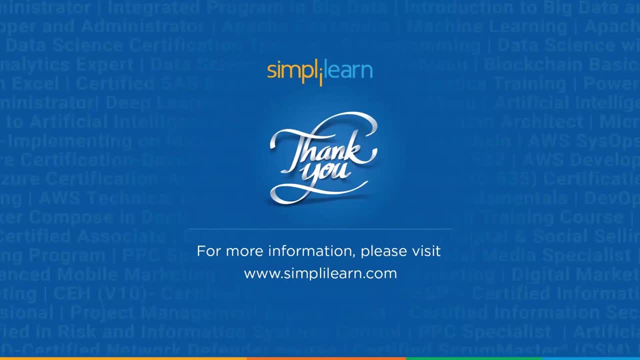 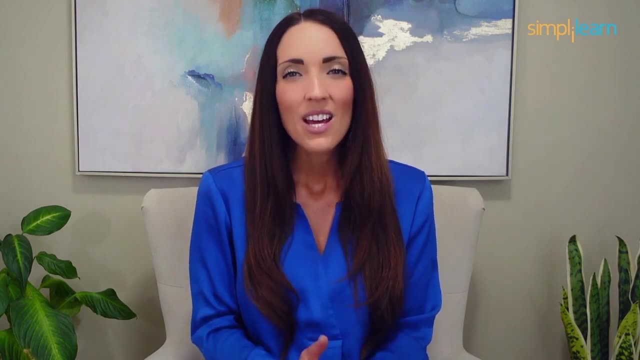 please give it a thumbs up. I hope it really helped you all. thanks for watching. stay safe and keep learning. Staying ahead in your career requires continuous learning and upskilling, Whether you're a student aiming to learn today's top skills or a working professional.